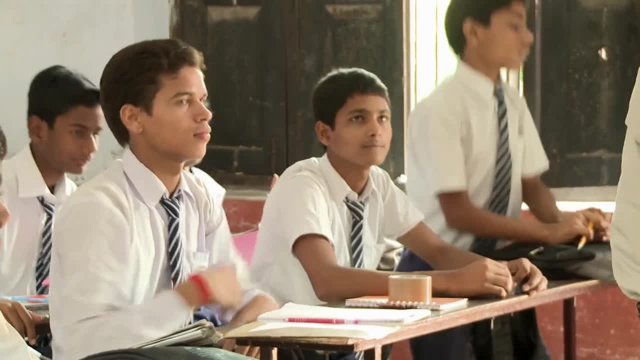 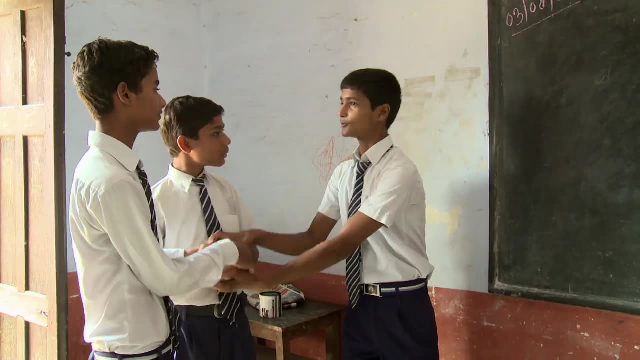 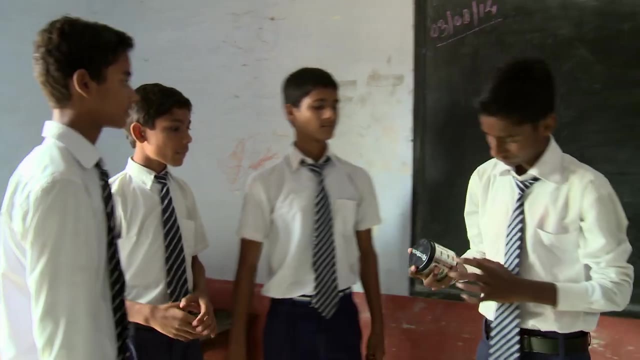 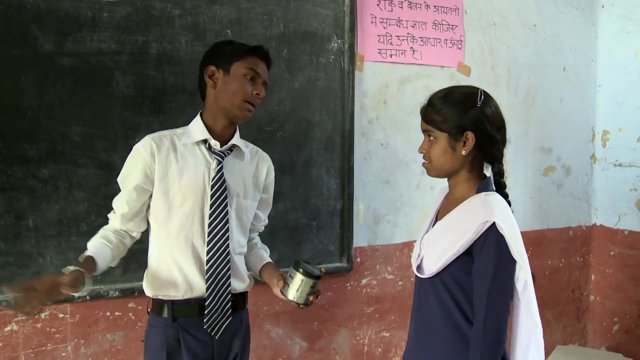 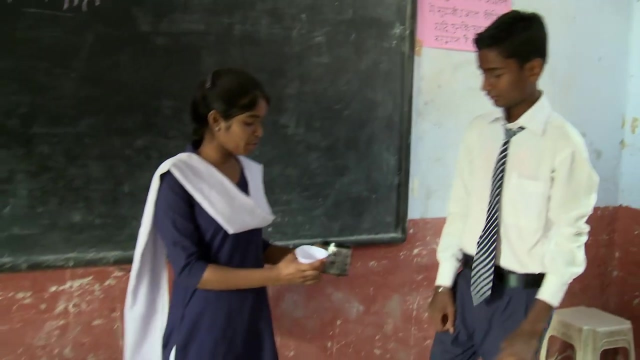 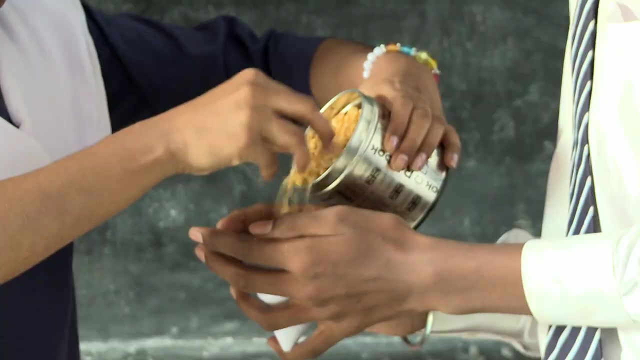 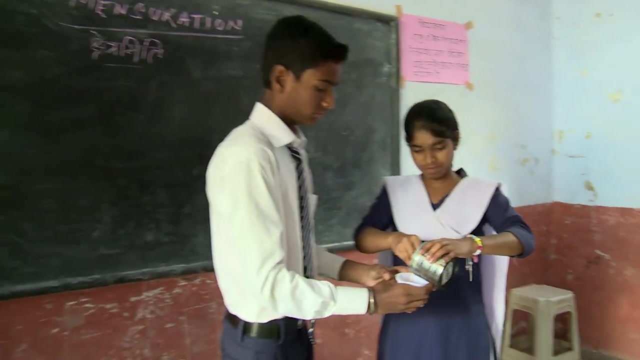 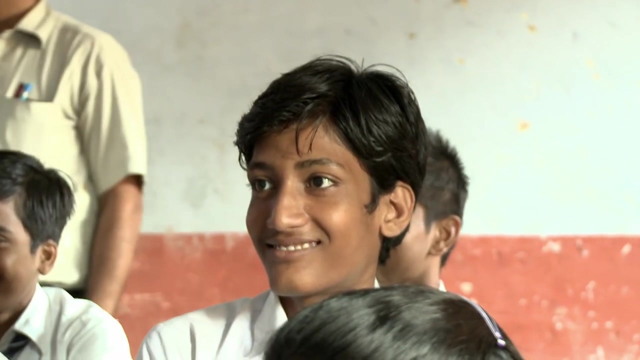 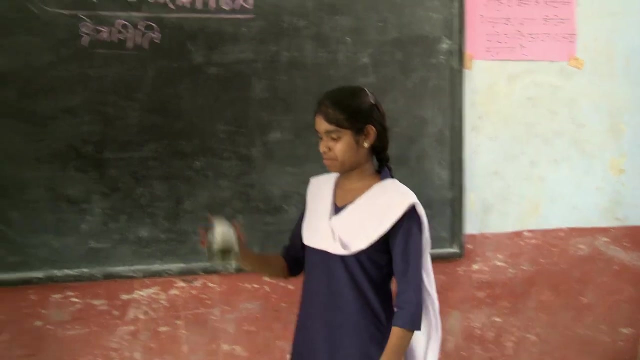 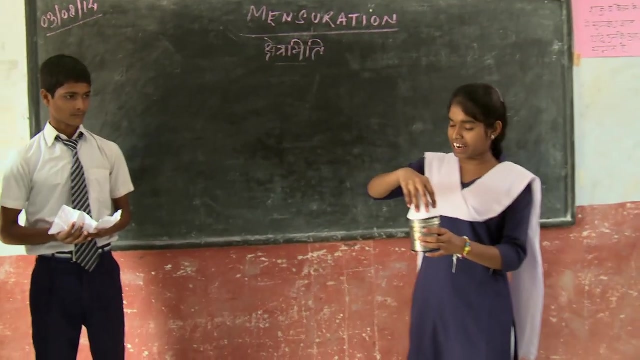 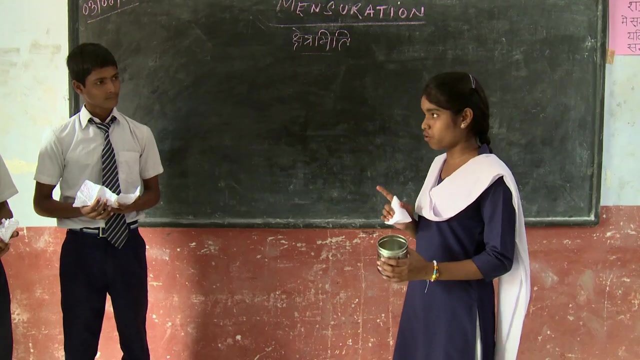 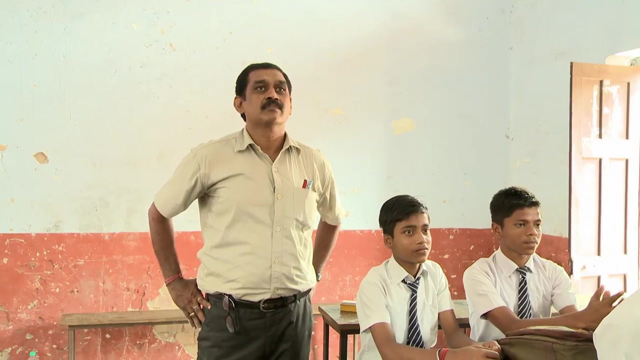 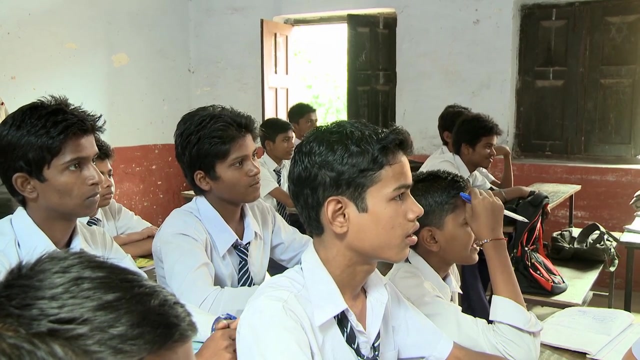 between the volume of a cone and a cylinder. Imaginatively, the students use a family dispute to illustrate the idea. This teacher has confidence in his students and trusts them, so he stands at the back of the class to watch the role plays. The teacher explains that group one has shown. 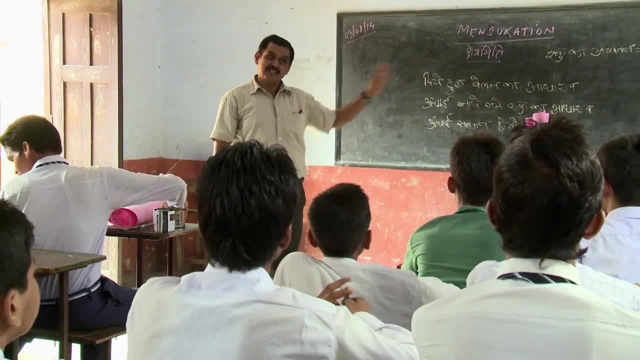 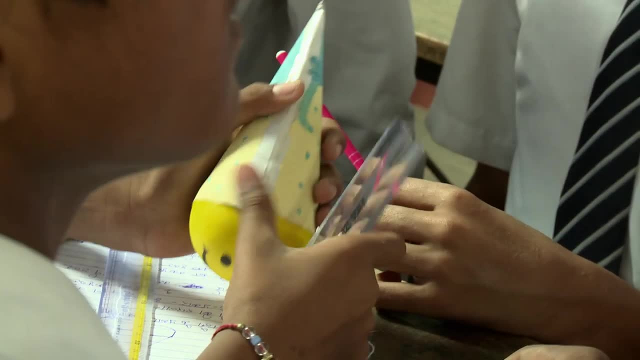 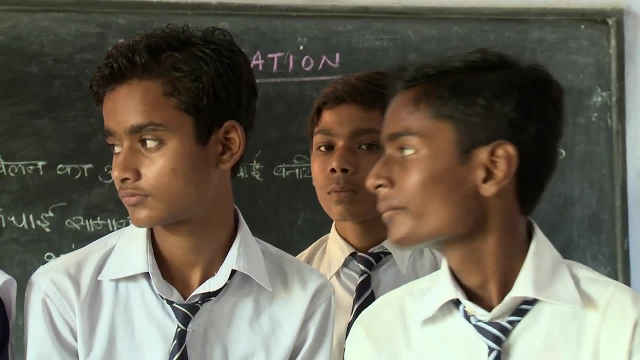 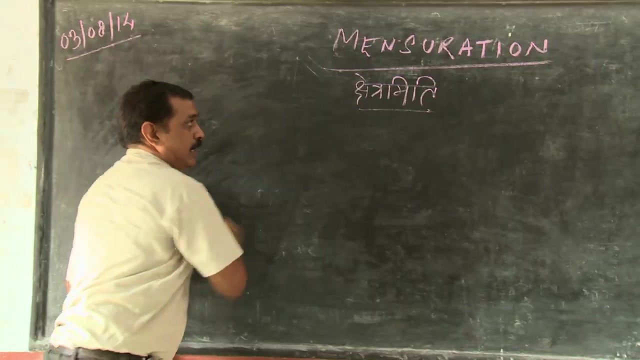 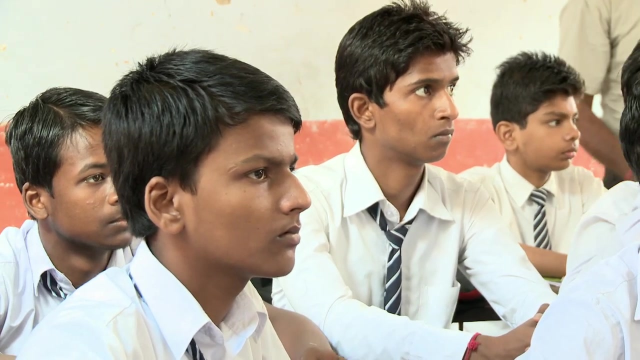 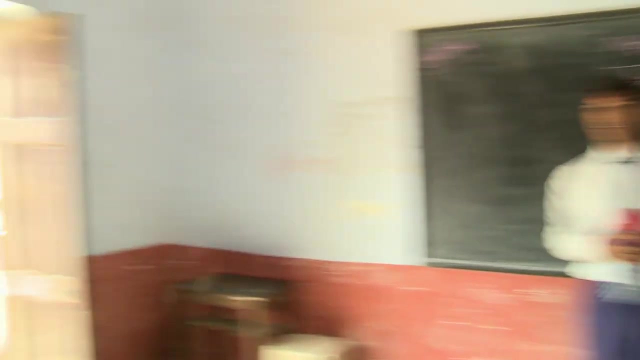 the volume of a cone and the volume of a cylinder. The teacher tells them that the counting of the cylinders is a position of diversity. The teacher says These role-plays provide opportunities for students to work in groups and for the teacher to assess their understanding. 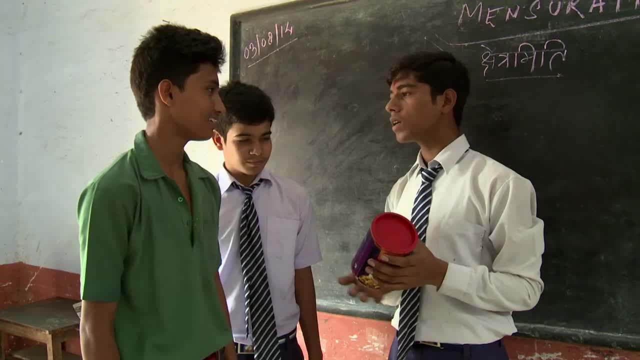 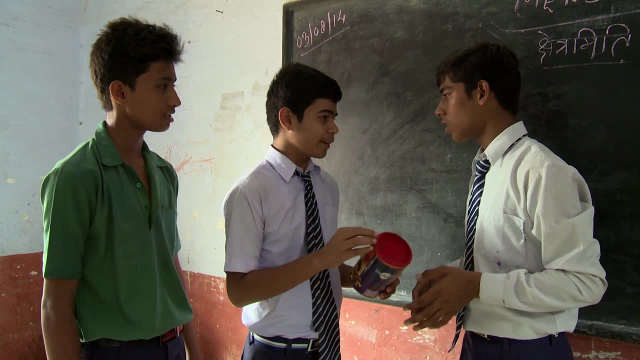 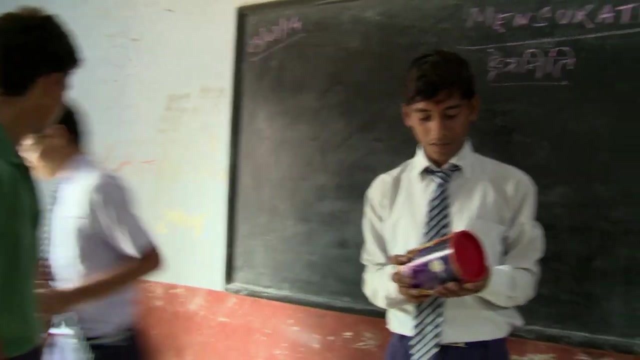 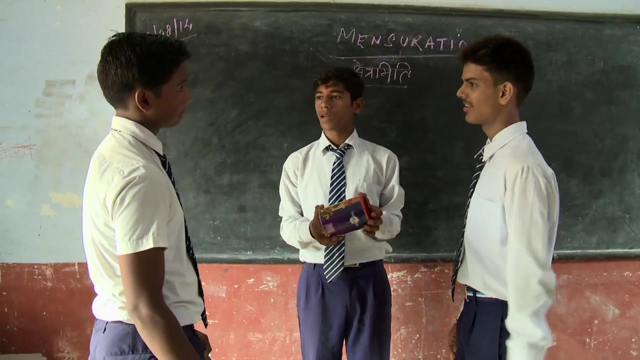 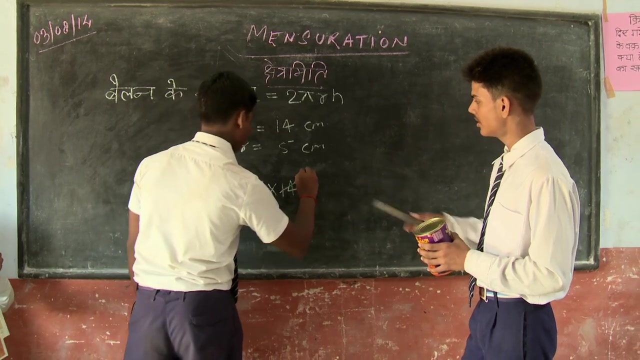 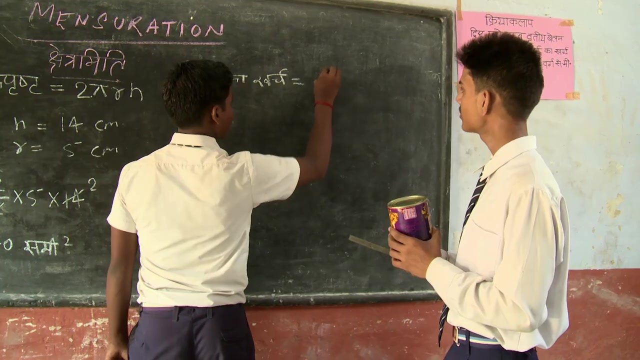 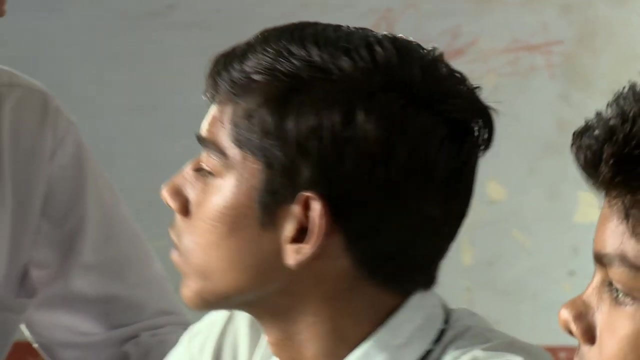 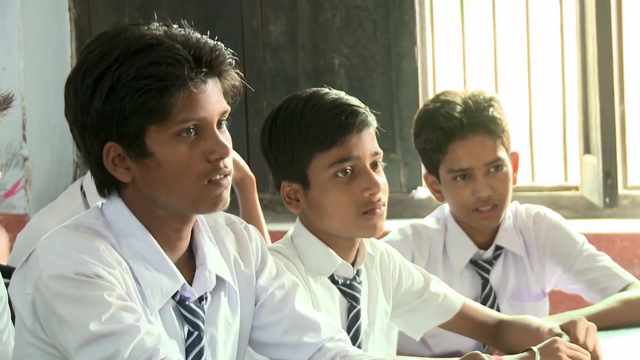 The next group presents a commercial transaction with a painter to illustrate their maths points. Afterwards the students describe how this type of activity helps them to feel more confident using maths outside school. The teacher encourages another group to present their role-play. One of the group enacts the teacher's role and instructs students to calculate the volume.